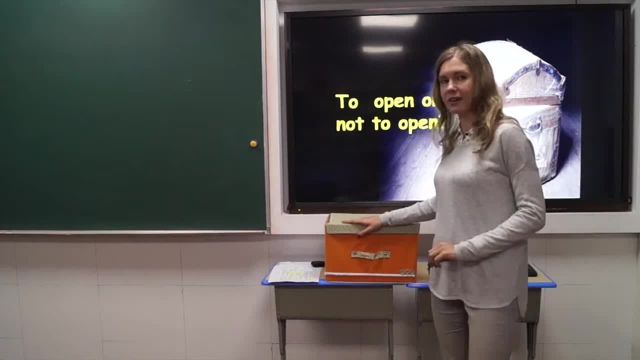 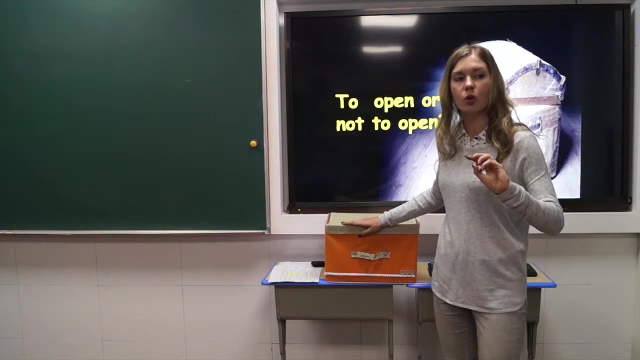 Yes, please, Oh yeah, maybe the dragons, right, I don't know So, but my question, the second question, was: who would like to open this box, Or maybe who wouldn't like to open this box? Now I want the people who really want to open this box to stand up. 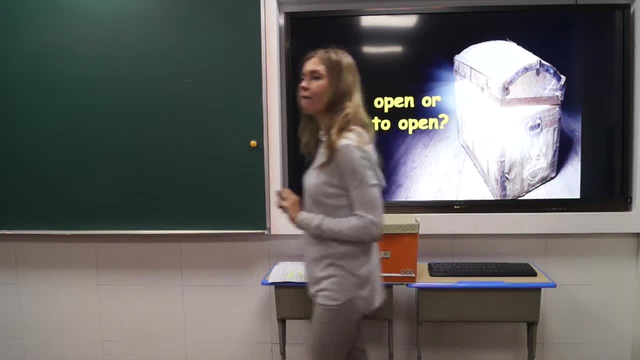 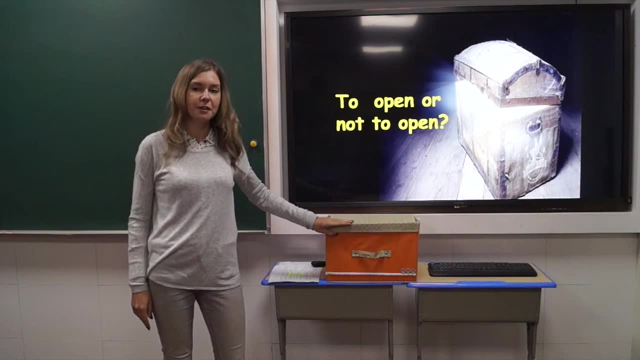 Mm-hmm, Let's see one, two, three, four, five, five people. So five people in the class want to open this box. Shall I do it. Okay, I think we'll leave this box till the end of the class. 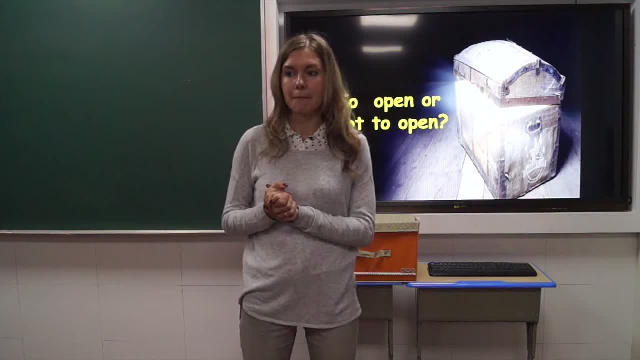 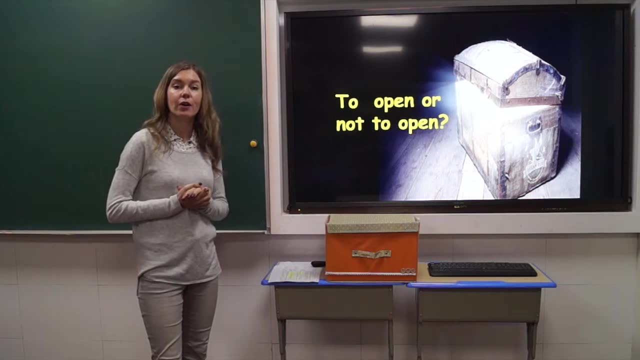 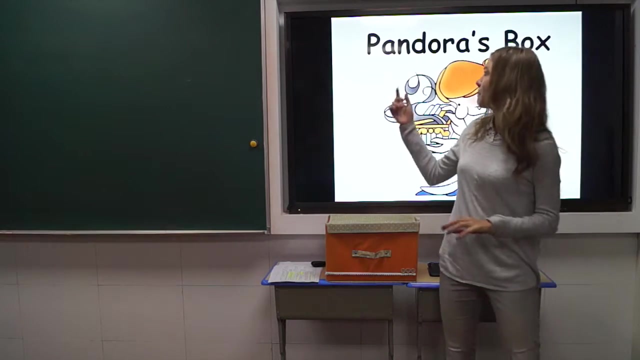 And then I'll ask you the same question one more time And we'll see what your answer will be. Okay, And at home I remember you read a story And do you remember what's the name of the story? Right, The name of the story is Pandora's Box. 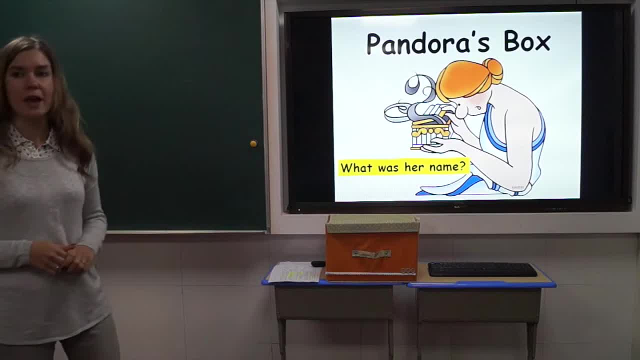 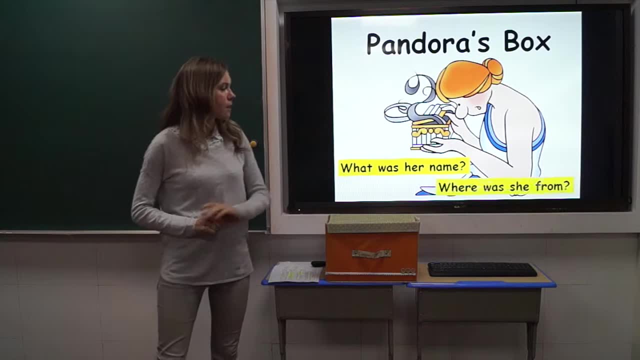 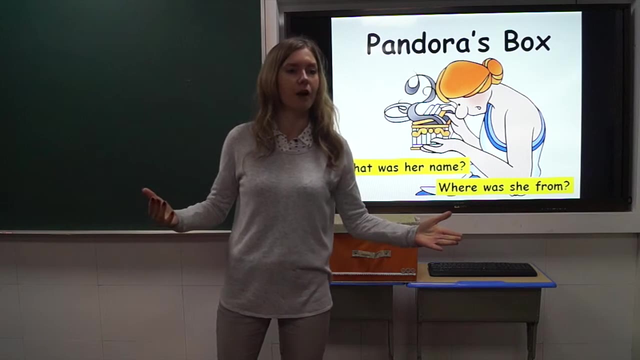 Okay, so what was her name? What was the name of this woman? Right, her name was Pandora. Pandora. Where was she from? Was she from China, Or Was she from America? Where was she from, Right, ancient Greece. 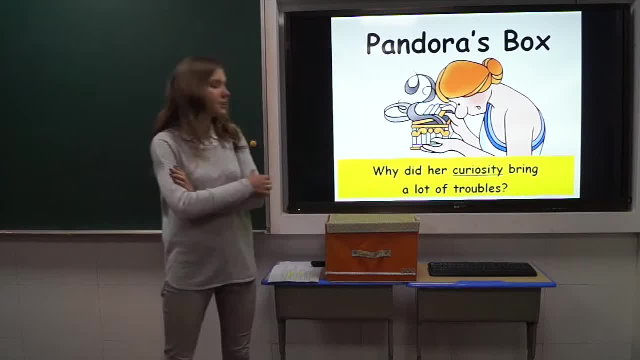 Athens. right, Good, And let's have a look at this question. Can I ask you to raise the question please? Why did your curiosity bring a lot of troubles? Mm-hmm, So was she curious? Was she a curious person? 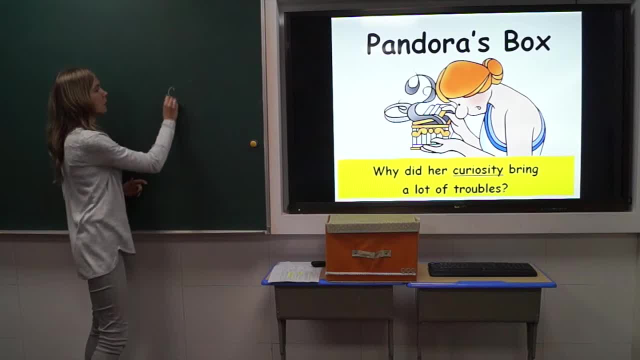 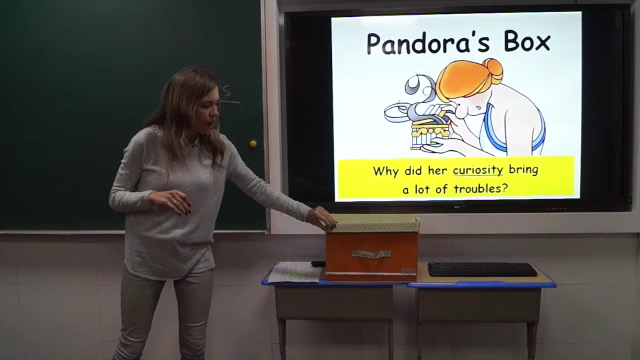 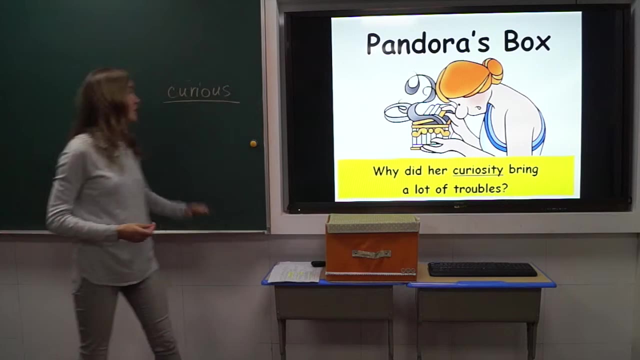 Let's have a look at the word curious. If I'm curious, would I want to open this box? Yeah, probably, because I really want to know what's inside. So being curious means you want to do something. yeah, You don't know what is it and you want to find it out. 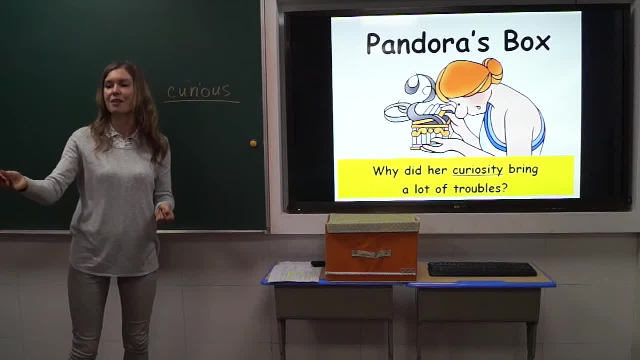 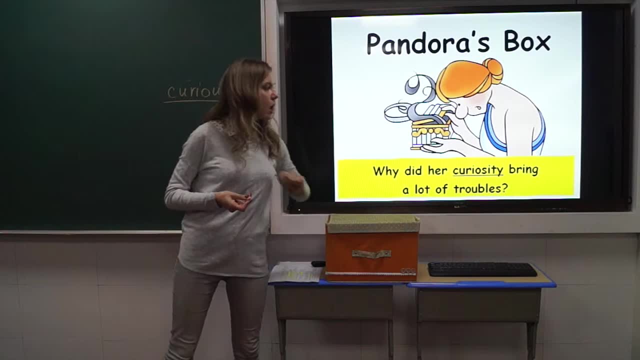 Are you curious? Some of you, yeah, I think all of us are very curious. Was she curious? Absolutely, She was very curious. So why did you open this box? So why did your curiosity bring a lot of troubles? 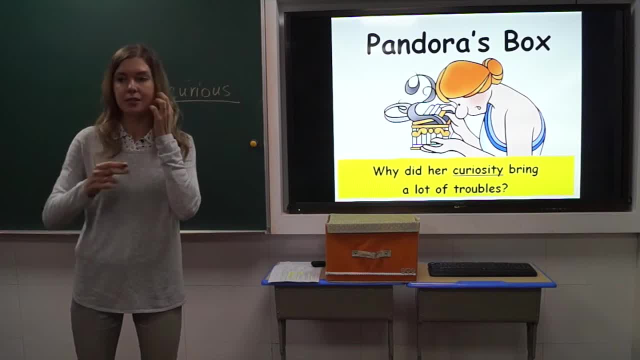 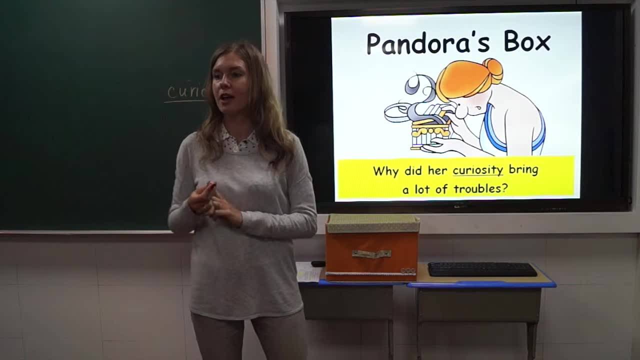 Yeah, try to remember the text you've read at home. I see some of the people haven't even opened the book. All right, you'll have a chance today to read the story, Okay. so yes, I think I will leave this question on the board. 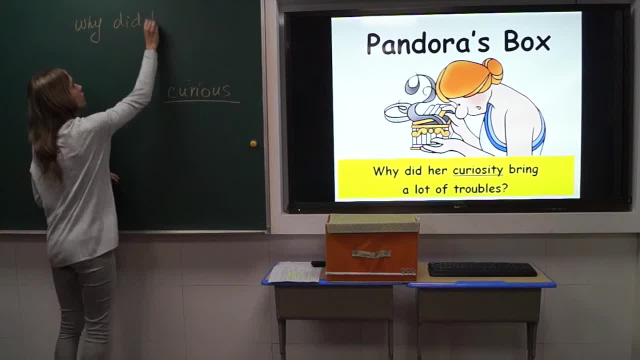 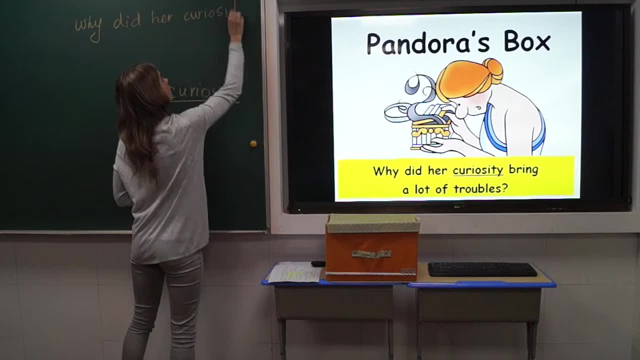 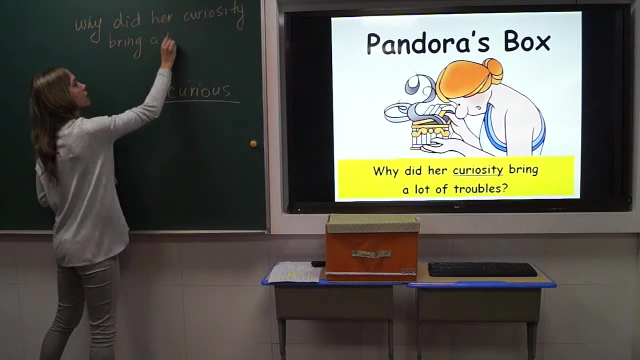 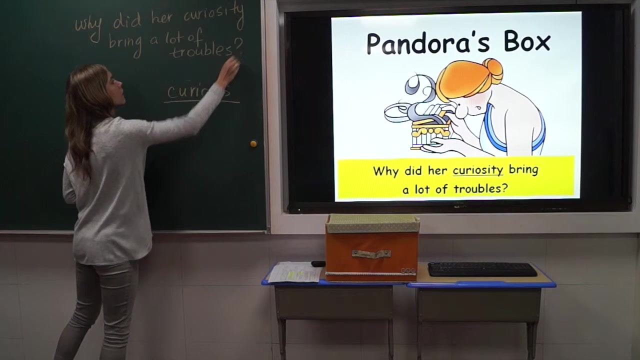 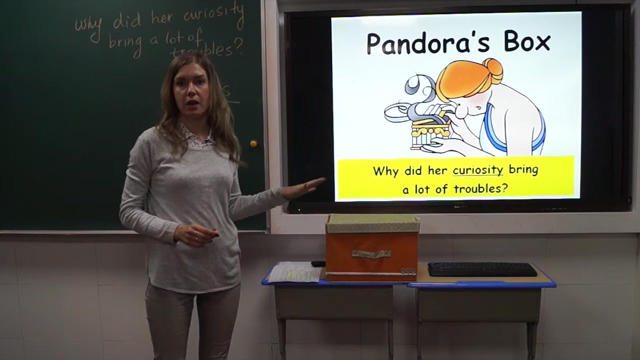 Why did her curiosity bring a lot of troubles? I will leave this question on the board and we'll try to go back to this question one more time at the end of the class and we'll see whether we can answer it or not. 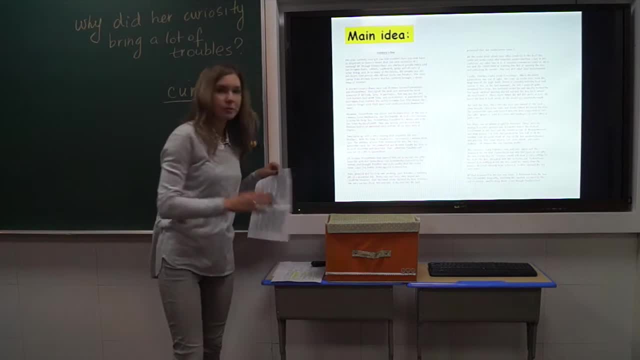 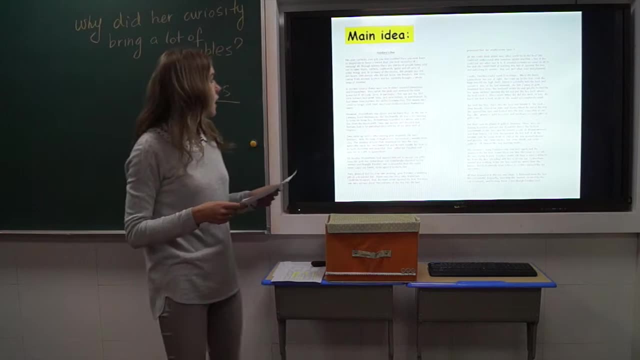 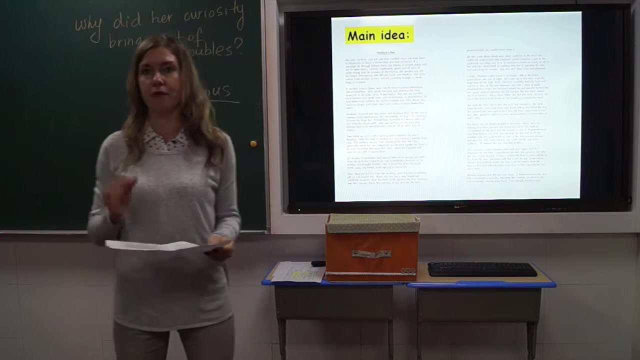 So at home, you read a text and I want you, please, to get your text ready, Find the worksheet I gave you yesterday and I want you to have a very quick look at the text and tell me what is the main idea of this text. 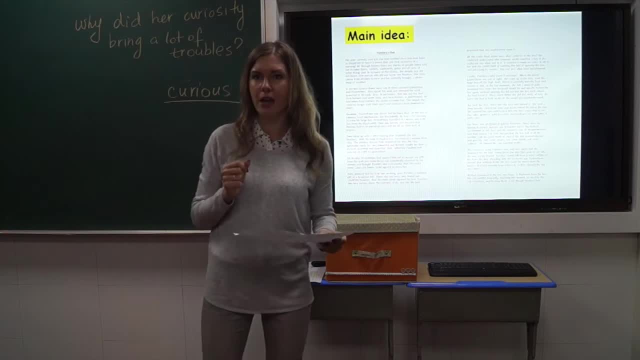 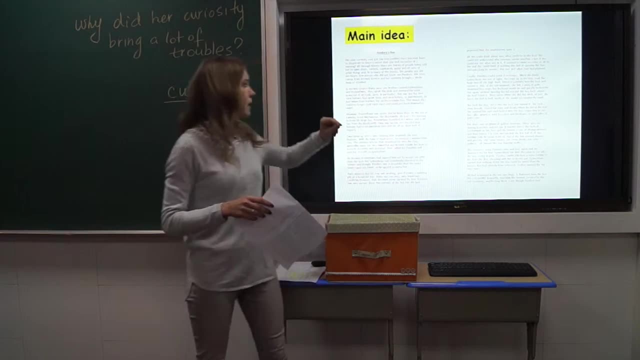 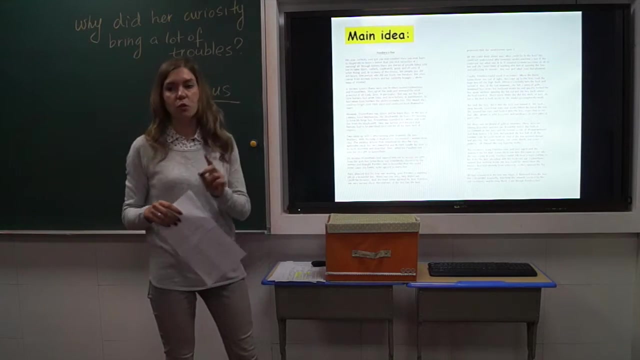 Please remind me when we're looking for the main idea. do we look somewhere in the center of the text? Not really? Where will be our attention at Exactly at the beginning, the first and the last paragraph, Right, Okay, so I give you one minute in pairs together. very quickly, try to think what is the main. 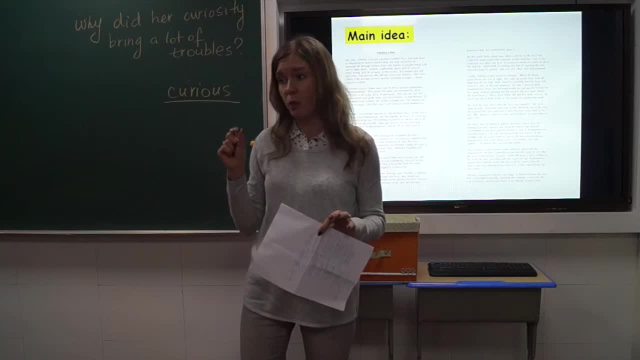 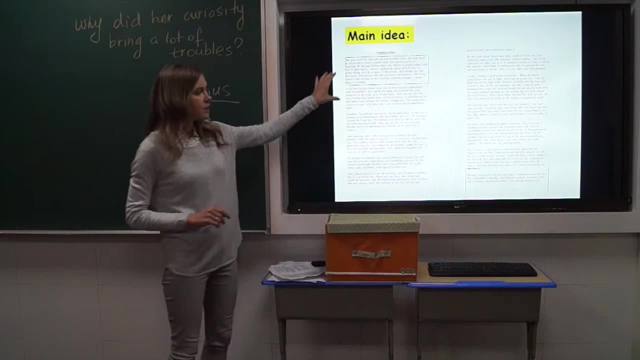 idea of the text And I remind you again, it should be one or maximum two sentences. Ready Go, All right, let's see. So let's have a look at the first and the last paragraph and what do you think is the? 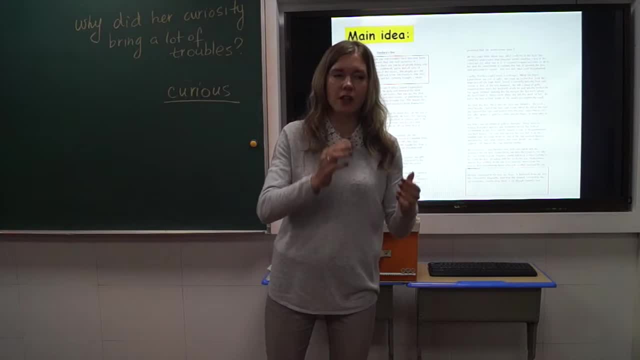 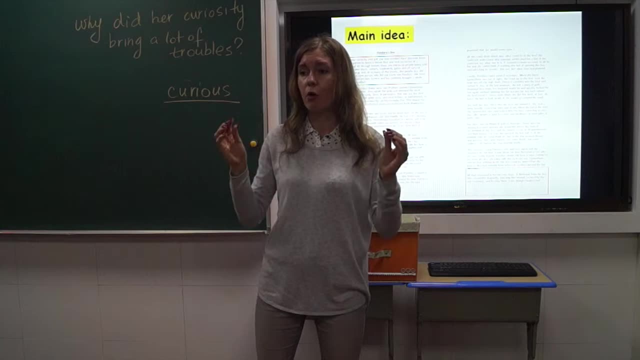 main idea. Okay, Nice, Try to paraphrase it. make a full sentence out of it. Remember: main idea should be formed in one sentence, not just a phrase or three or four words. Make a sentence, guys. Aha, what is the main idea? 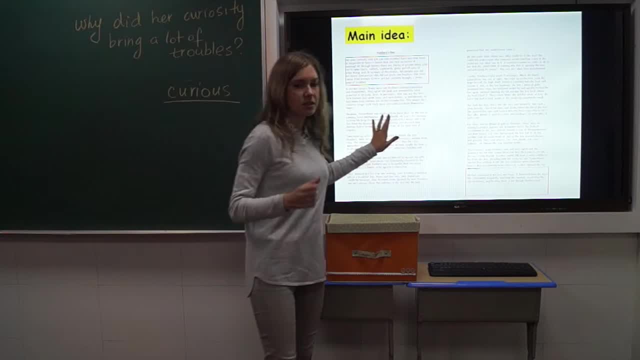 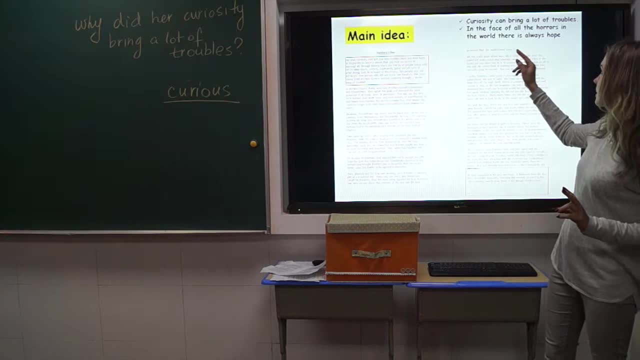 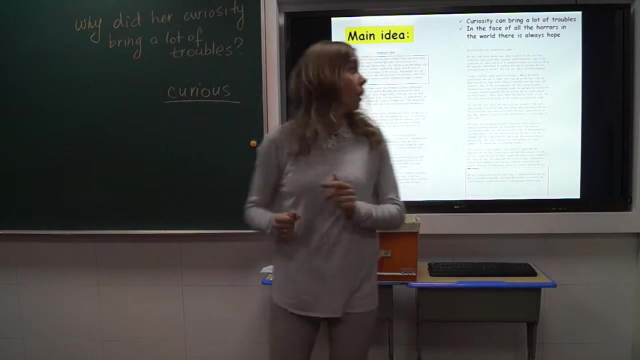 Interesting. Okay, so let's summarize it very quickly. So this text has actually two main ideas. We can say that curiosity can bring a lot of trouble Right And in the face of all the horrors in the world, there is always hope. 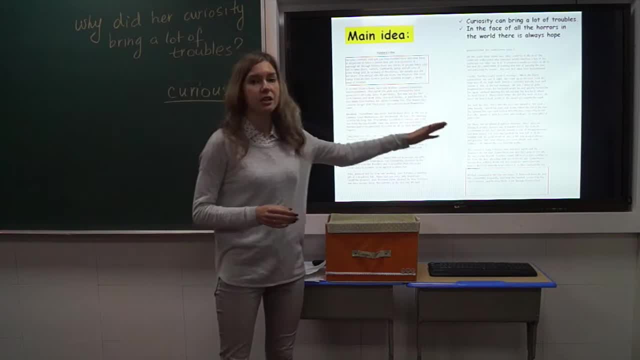 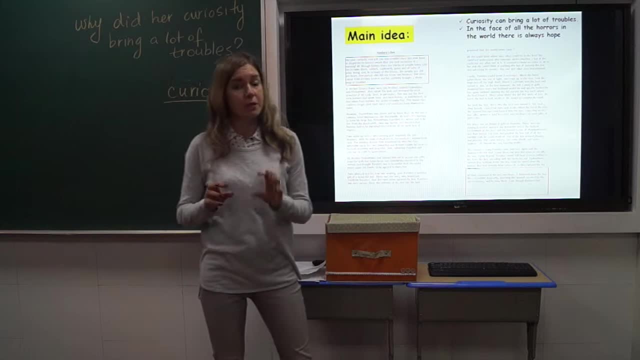 Yeah, you might have noticed that these two main ideas are in different places. The first one is in the first paragraph and the second one is in the second paragraph. We still would keep them both. sometimes it happens the text has two main ideas. 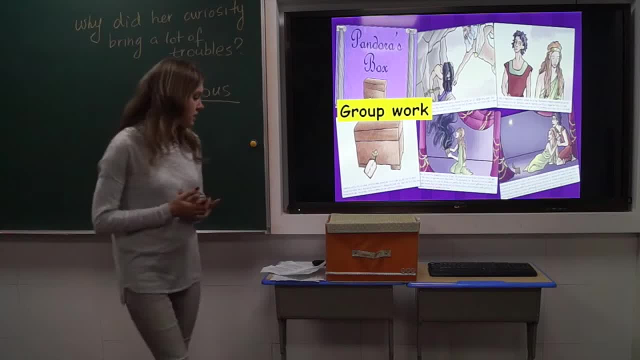 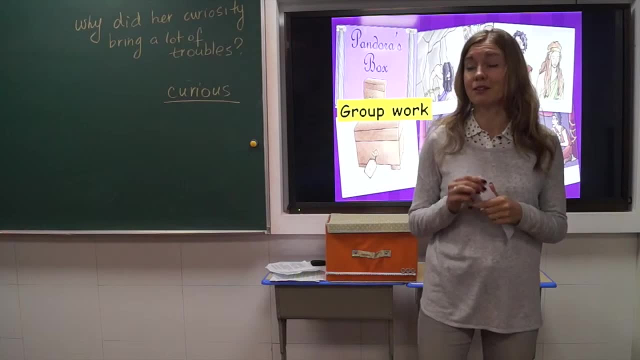 Okay, Good job everyone, And now let's move on. Let's remember how well, how well, how thoroughly we read the story. So, right now, each team. let's have a look. we'll have a team of threes today. 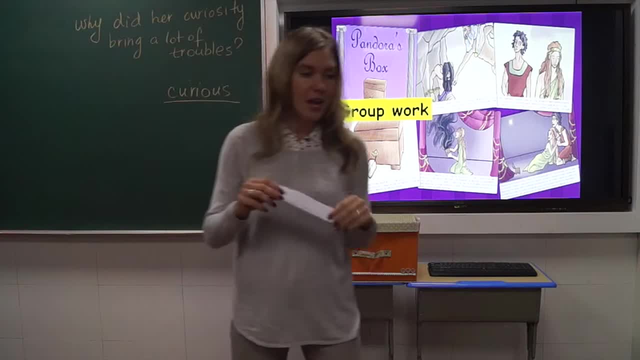 You three, you three and you three together. Okay, Each team will be given a set of cards with the sentences on them. These sentences are the extra extracts from the story. How many sentences do you think? I have Exactly 12 sentences. 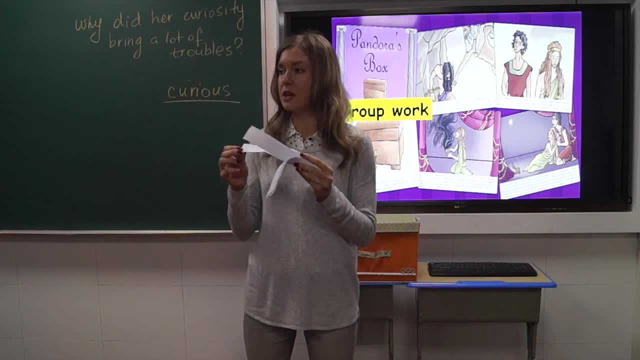 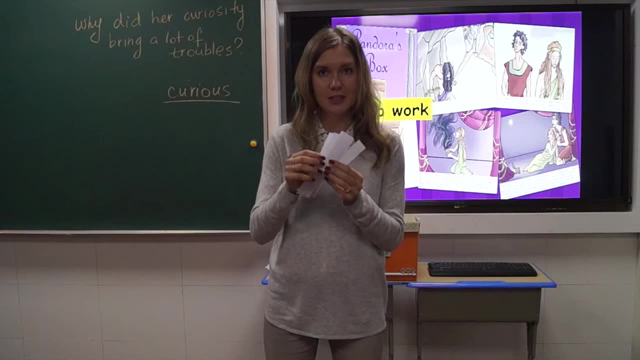 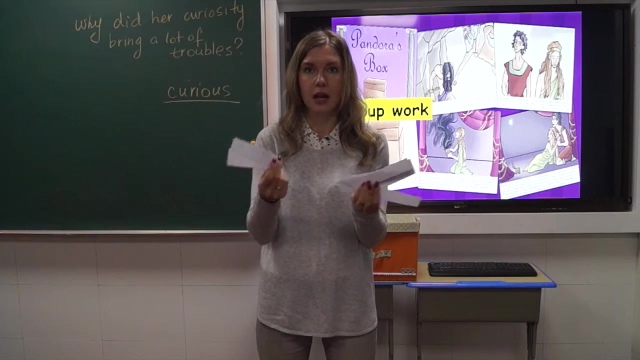 It means there are 12 ideas from the text. What do you think you should do? Do you need to read the sentences? Absolutely, But you see all the cards. they're jumbled, They make no sense. It means in pairs, in threes. you need to put the sentences in the right order from. 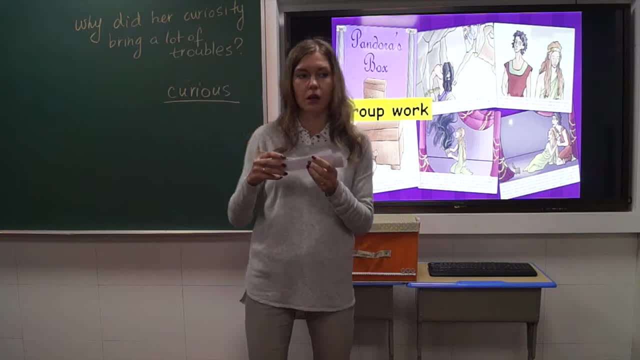 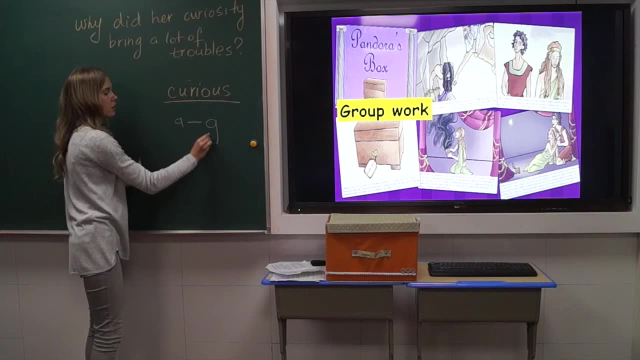 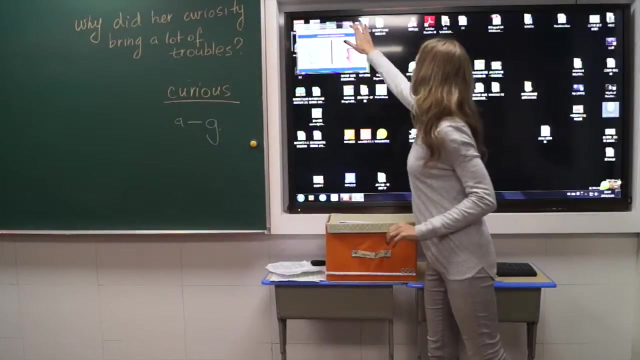 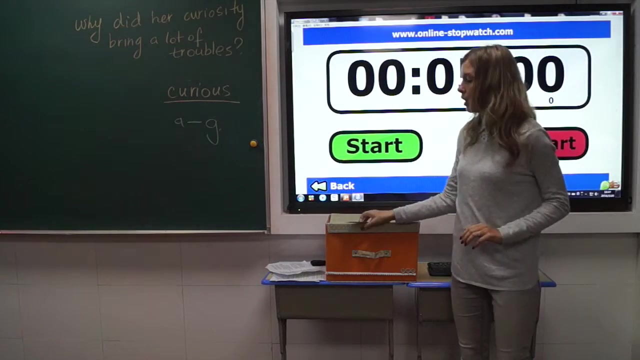 letter A And then you put the other words from letter B, From letter A to letter G. You can clear your desks first and get ready for this activity. Okay, Five minutes should be enough. Remember, you read the sentences. Do you write letters or numbers? 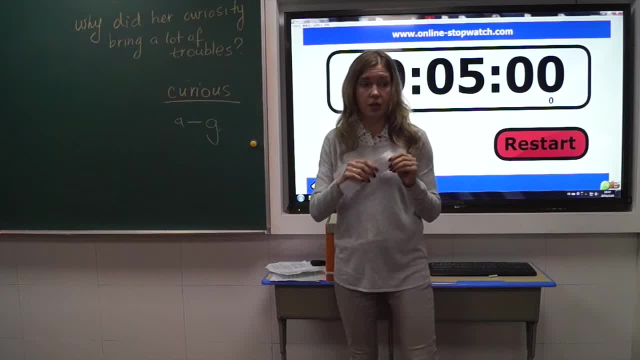 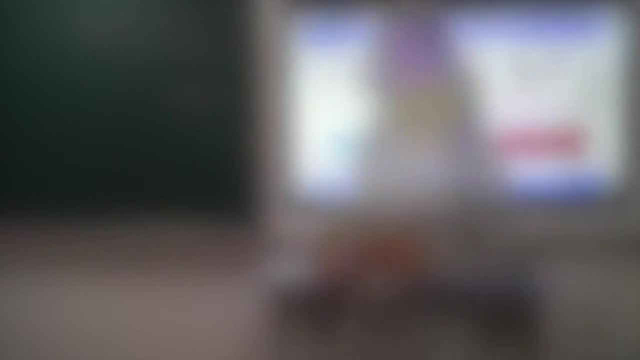 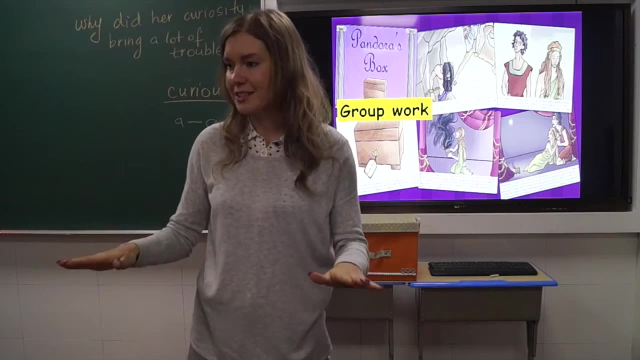 Do you actually need to write anything? Not really. Just read the sentences and put them in the right order: Ready Go. Okay, let's go back to our story Now. you have all the cards on your desks And I already asked team number three to come on the board. 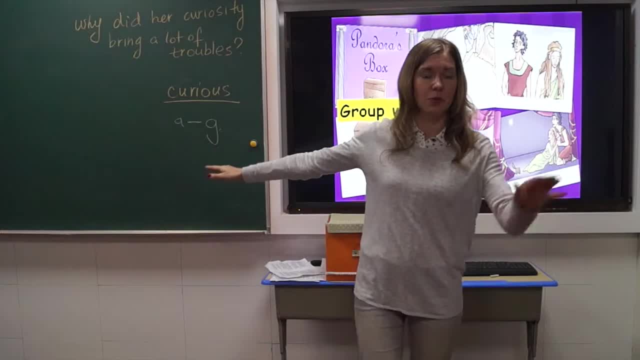 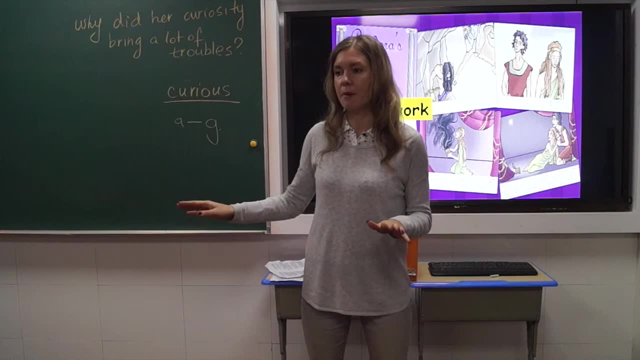 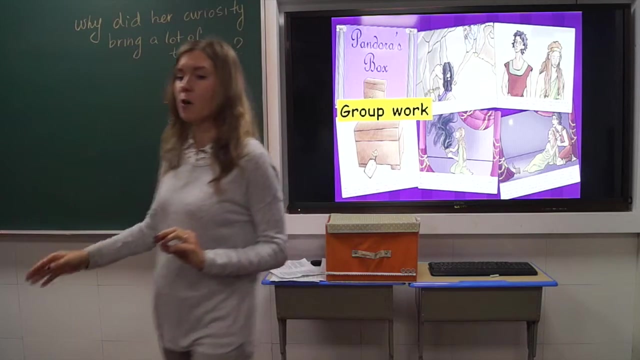 Please look at the answers and check these answers with the one your team had. Please raise your hand if you have different answers. Good job, So everyone has the same Well done. Well done, Okay, excellent, excellent. Now, please the team leaders collect the cards and put it on my desk. 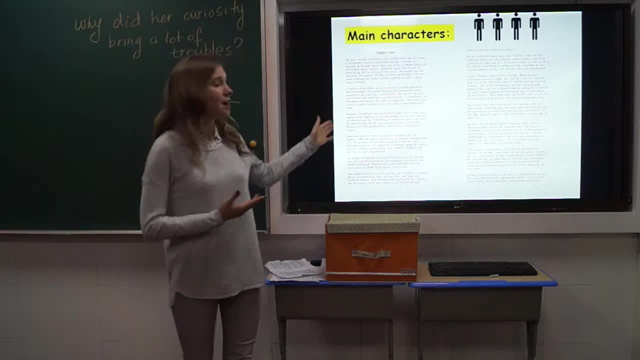 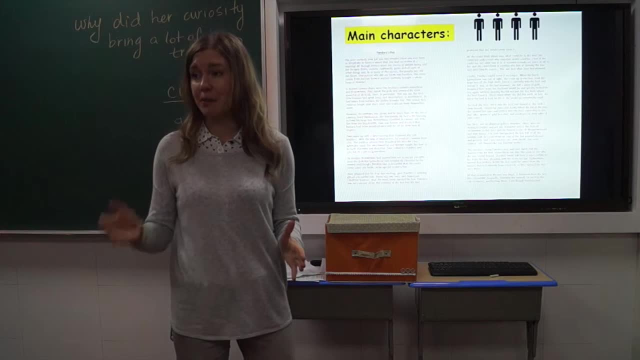 Thank you very much. Okay, Now it's time to move on. As we usually do when we read the story, we'll try to talk about the main characters, Because these are the people who are extremely important And they influence the whole gist and the whole idea of the text. 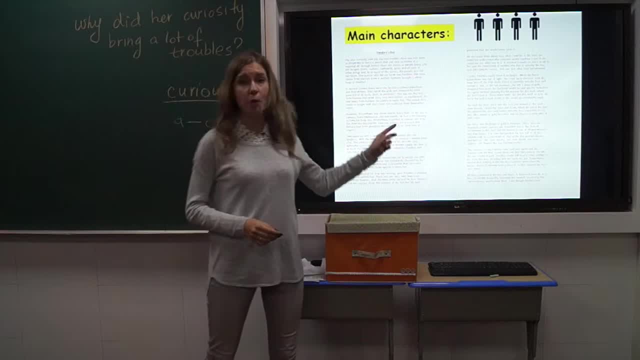 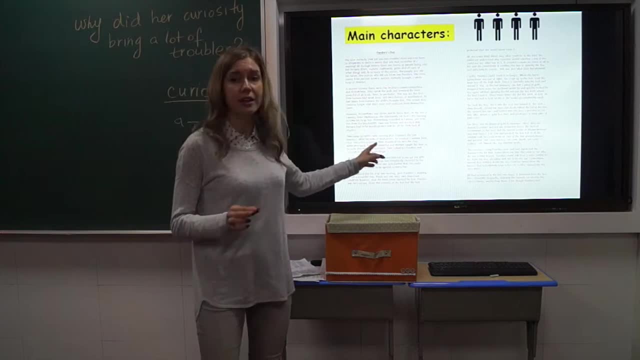 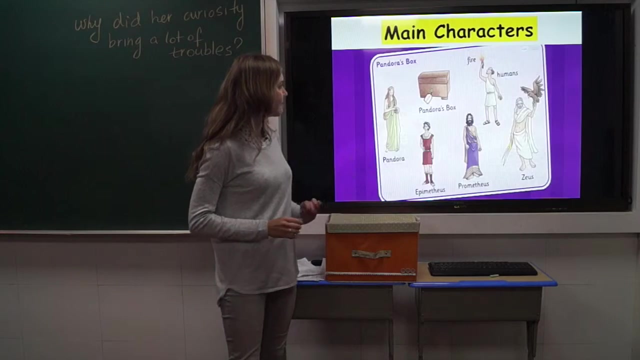 Now you've read the story. It's a very short story, but it has four main characters. Now I give you two minutes in pairs. Try to underline the names of the main characters. Ready, Go, Okay, And now let's check everyone. 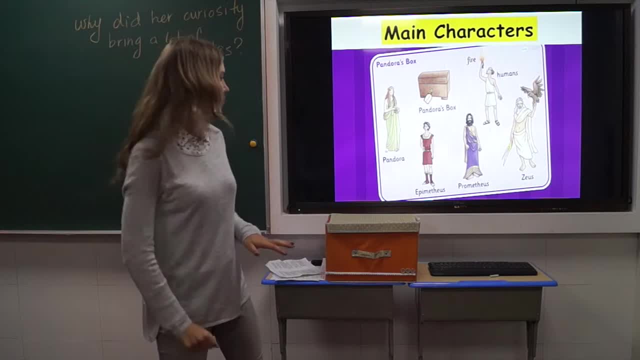 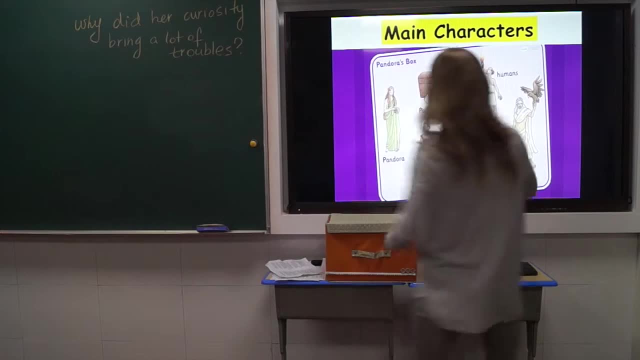 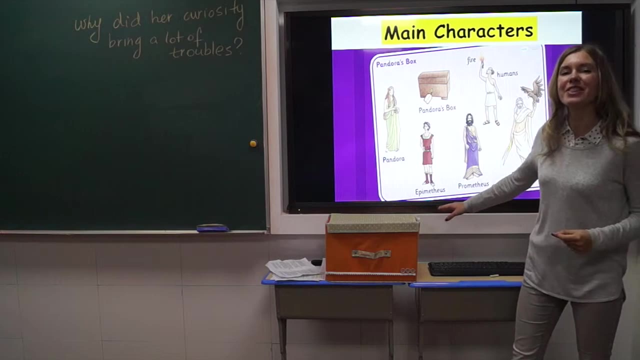 So I think you all noticed that there are four characters. And what is the first one? Pandora, Right, right. How about the second one? So Repeat after me: Epimetheus, Epimetheus. Okay, now this team. 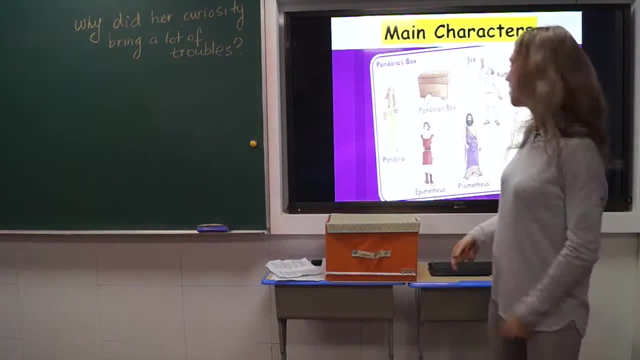 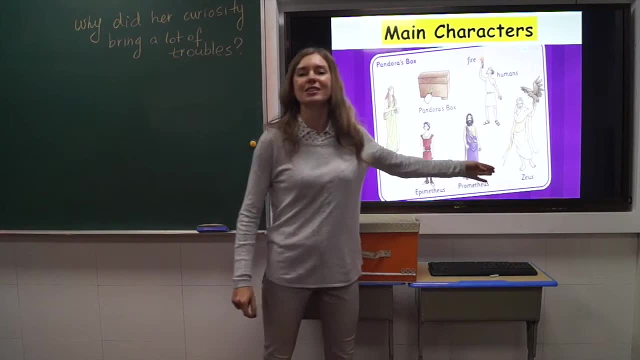 Epimetheus- Epimetheus Right Prometheus- Prometheus Good job. And Zeus Good, Zeus Excellent. So these are the four main characters. You might notice that their names are very repetitive in the text, So I'm going to read them one by one. 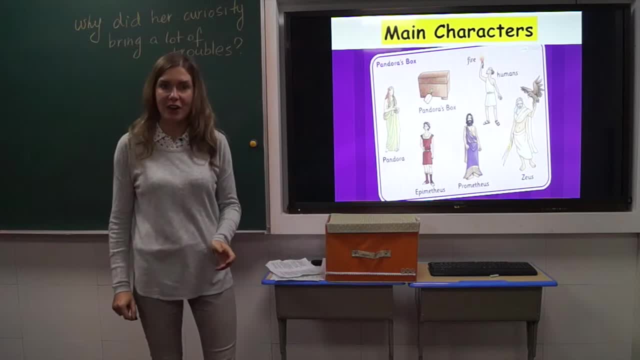 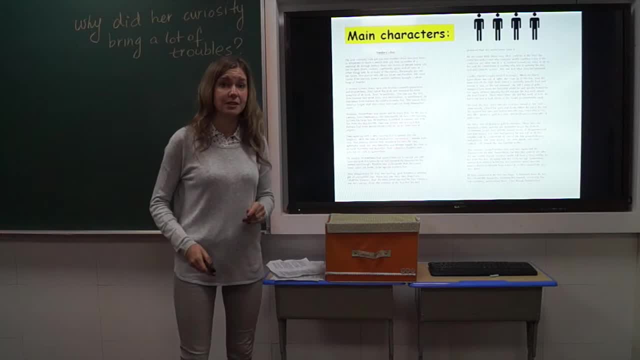 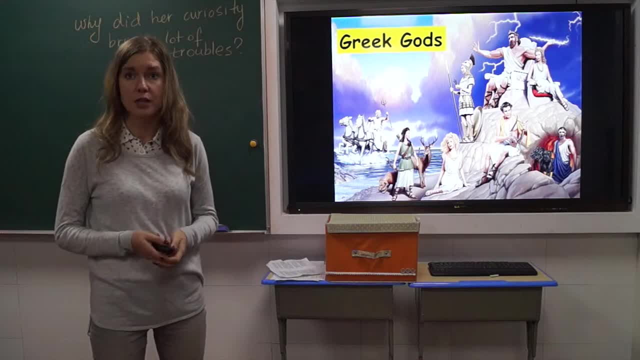 Uberäm, Uberäm. Do not forget the hoorah Uberießen. You might notice that there are some other Greek gods here, And in Greece they did have a lot of gods, And I will stuff that into our text. and can you name Greek god, right? 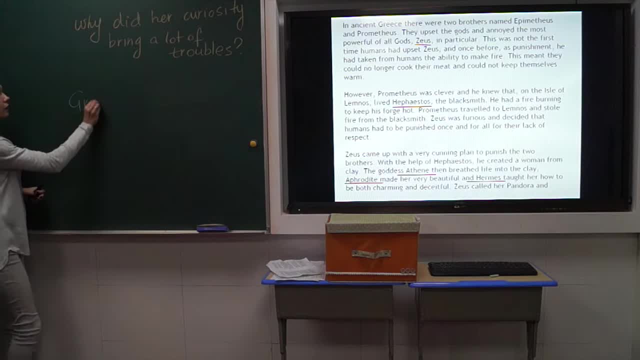 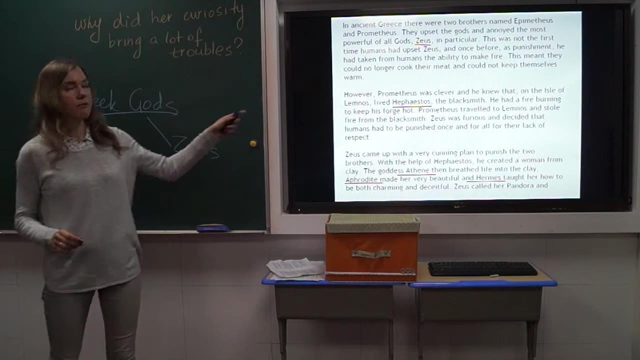 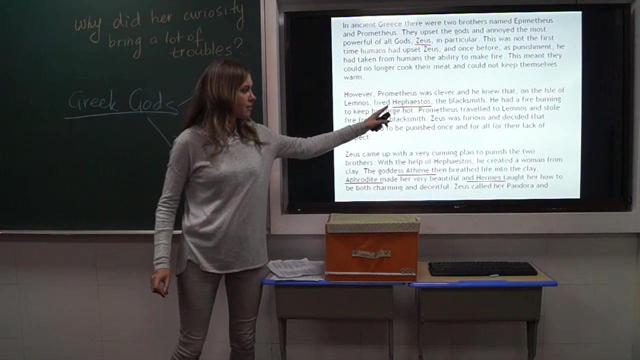 I want him to. So the first one. you already said his name is Lord, Lord, Lord, Lord Zeus. His name is Zeus. What are the names of the other Greek gods you could find in the text Right? a very hard name to pronounce, absolutely: Hephaestus. Okay, repeat after. 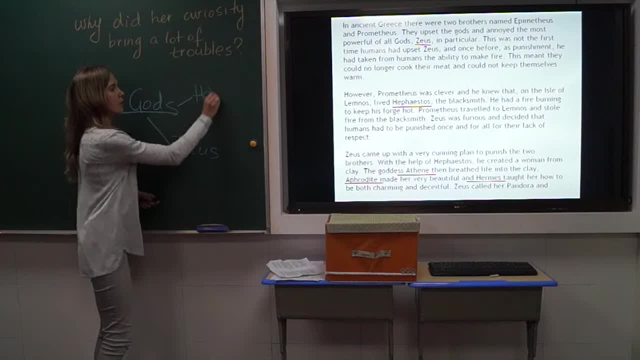 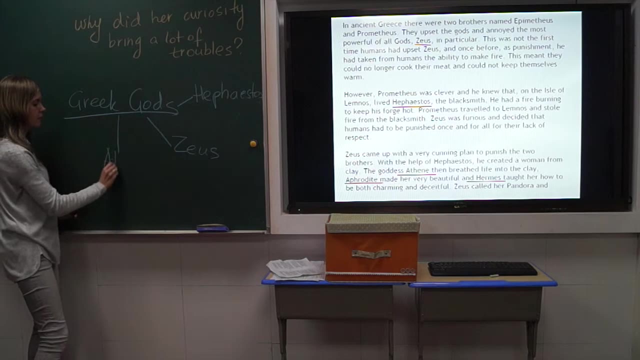 me, Hephaestus. Don't waste your time. Have a look at the third, fourth paragraphs and find some other names here. Okay, so the next one is Which one? Yes, Athene, Athene, Good. And the next one is Aphrodite, Absolutely Aphrodite. And there is one more. 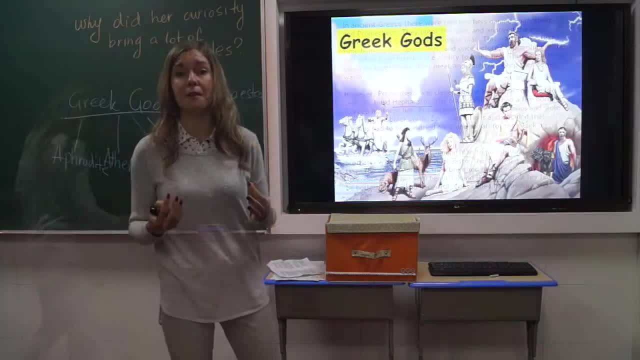 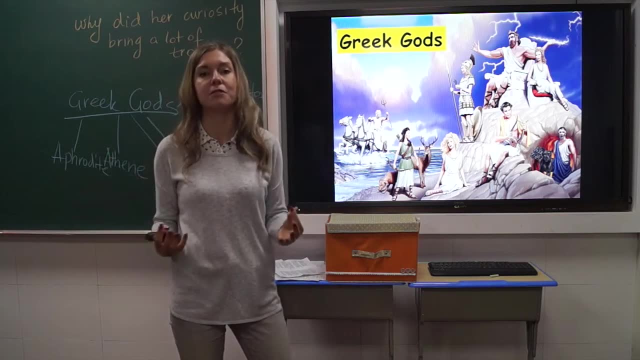 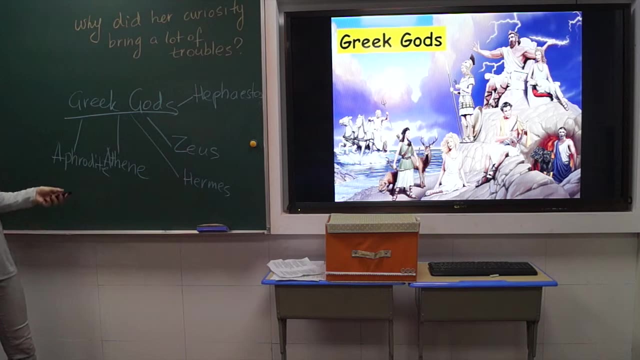 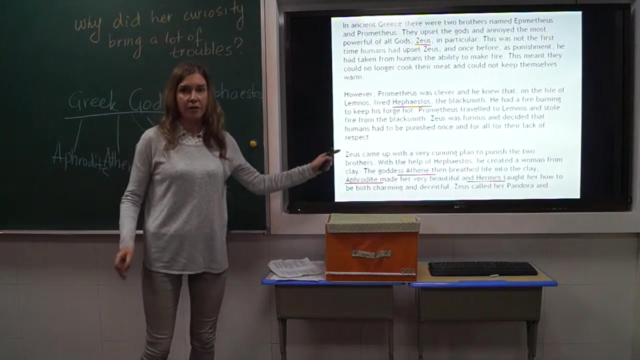 Godless. Good job, John. of hunting, of time, of death, of birth. of different gods have different domains. Now, looking back at the names of the gods you've mentioned, I want you to try to guess what are these Greek gods' domains? Again, looking at these paragraphs, 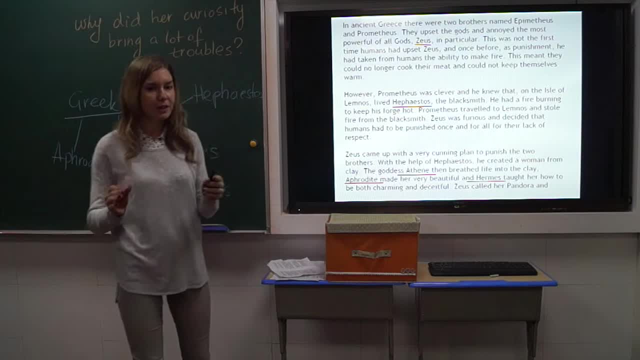 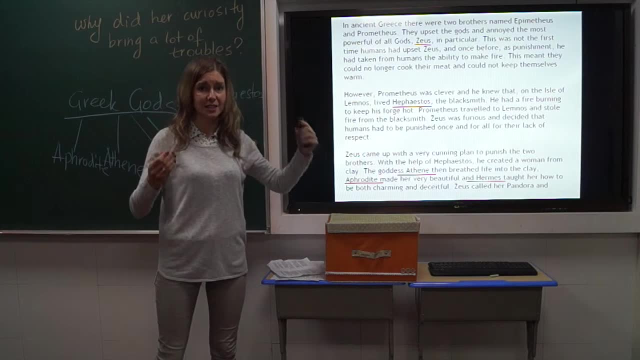 might help you Very quickly, very briefly, look at the text and try to think. Look at the Zeus first. Find some information about him and try to guess his domain: Mm-hmm, Exactly, It says that he is the most powerful of all gods. So he is the leader. Yeah, He. 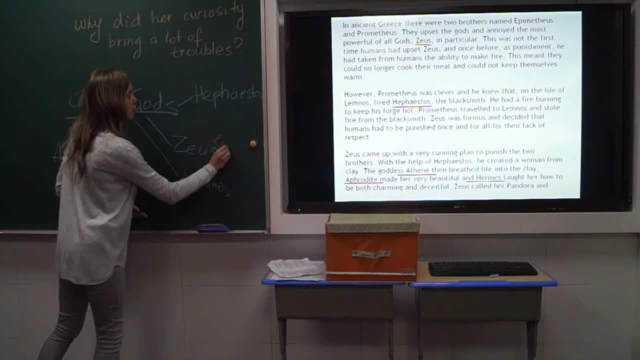 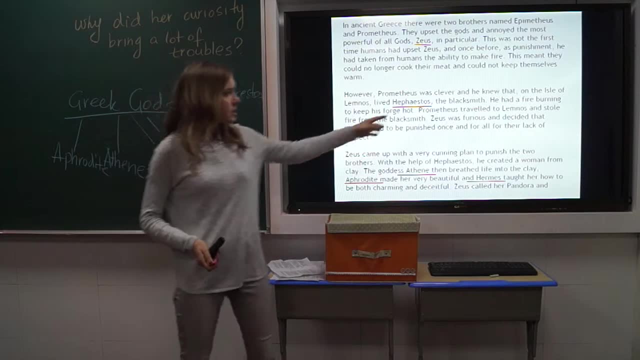 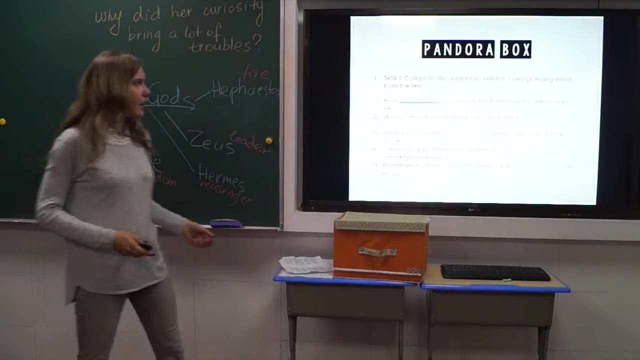 is the leader or the father of all gods, Excellent. How about Hephaestus? Uh-huh, Excellent. So he is the blacksmith. So if a person is a blacksmith, What does he do? Okay, good job. And now, guys, right now, I'll give you the handout. 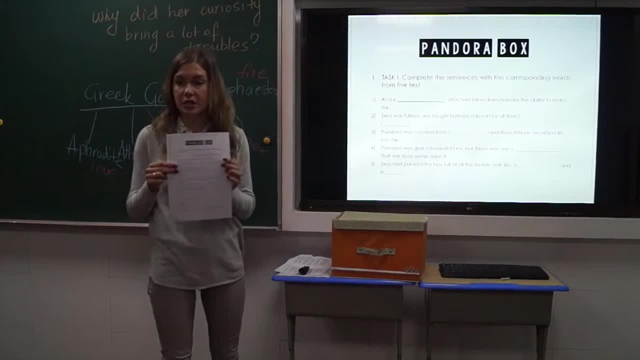 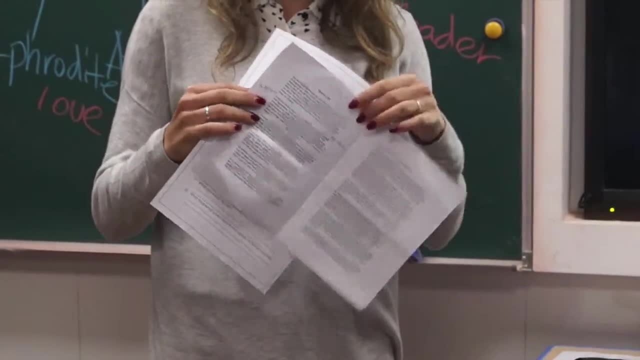 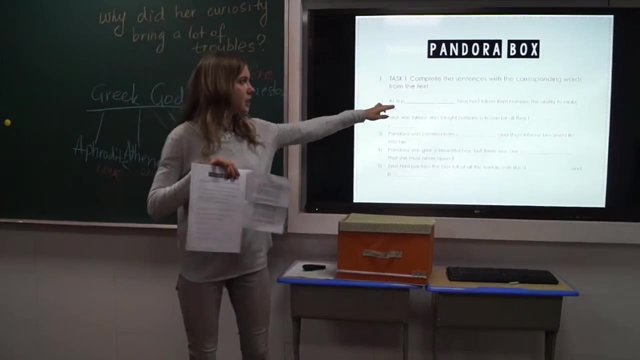 I want to have a look at task one. This is an individual work. Please refer to the text you've read at home. You can use the story to help you And finish the sentences one, two, three, four and five. What do you need to write in here? The words. 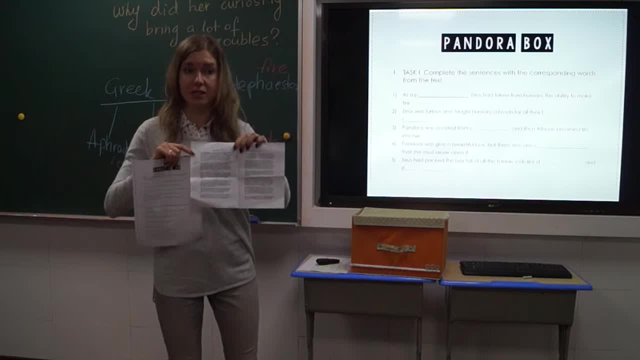 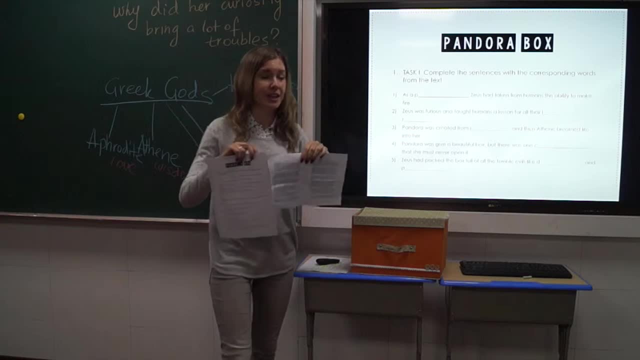 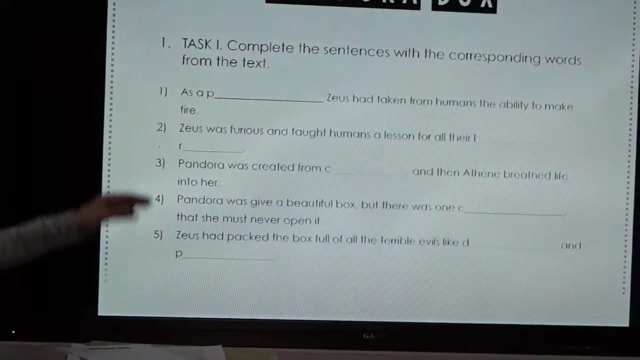 Where can you find these words Exactly In the text- And there is a great help here- The first initial letter of the word Exactly. Good, You have about three minutes. Okay, You can start right now And let me check the first sentence. The first sentence: Any. 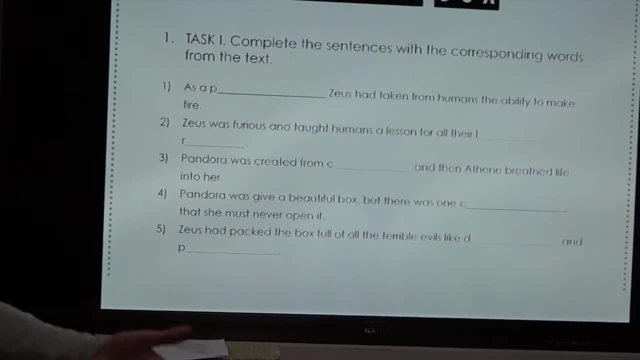 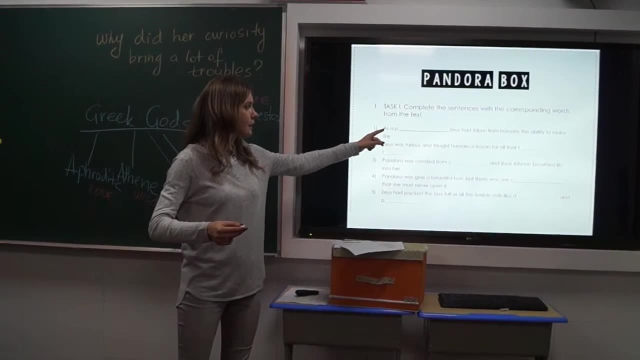 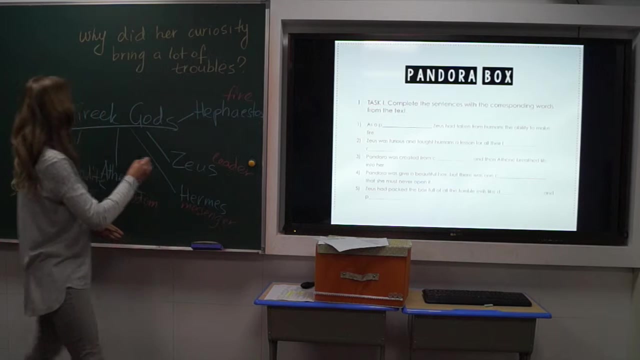 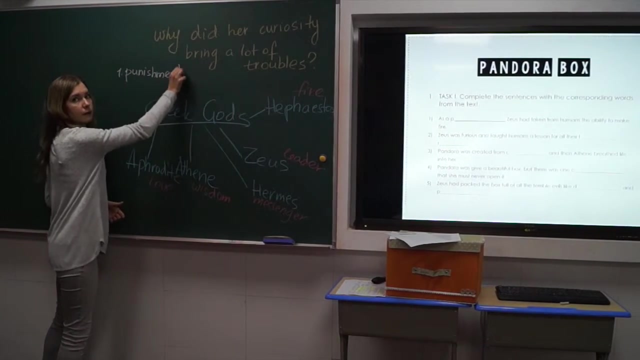 volunteers to answer this team? Please two people. I want you to stand up and read the question. the sentence together: Ready Go, Uh-huh, Exactly. So what is the correct answer? Number one is punishment. Good job, Okay. 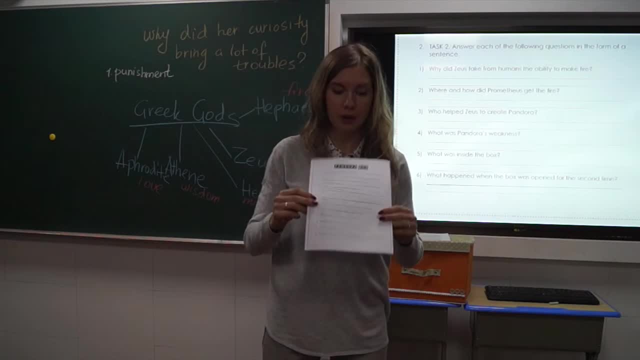 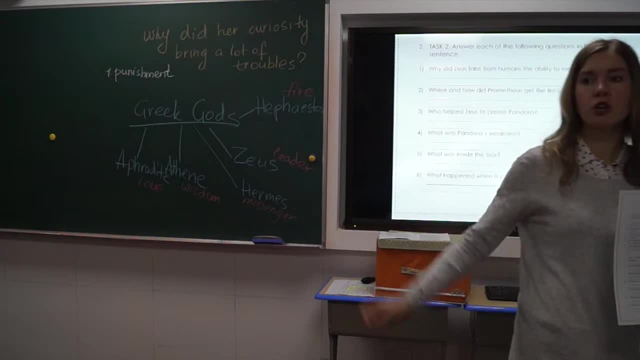 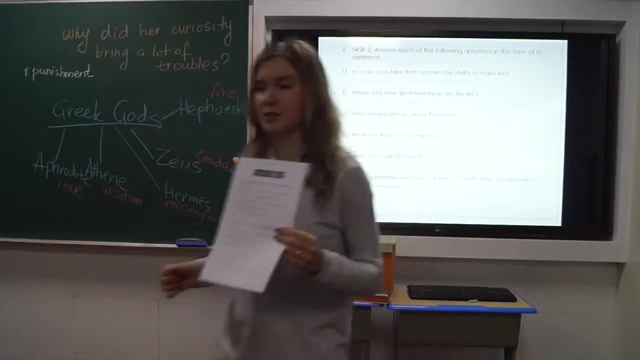 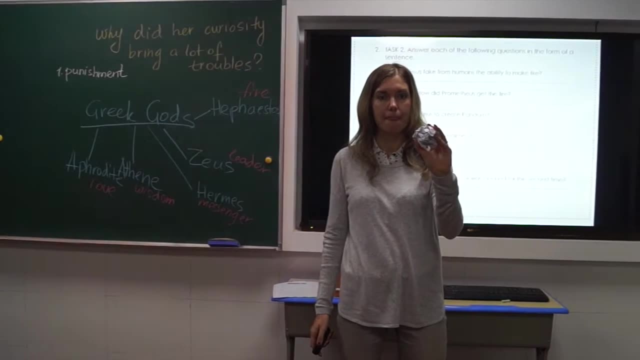 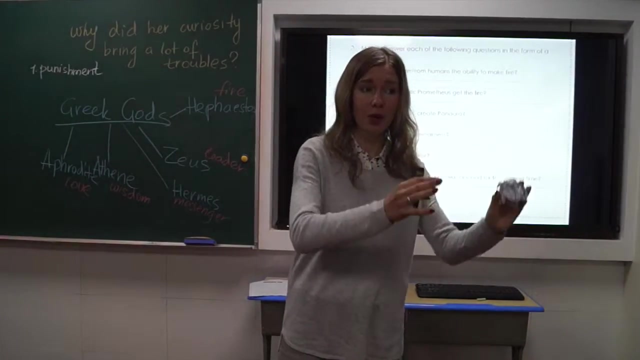 word. No Full sentences, guys. That's very important. Ready, Go Now. let's have a look. I have a ball of paper here And right now we're doing that as a whole class. Everyone will pass the paper from one student to another When the music. 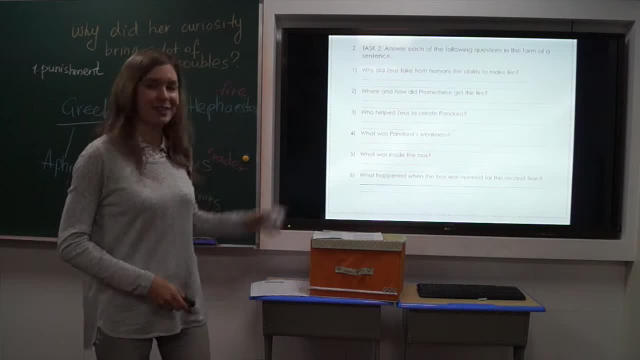 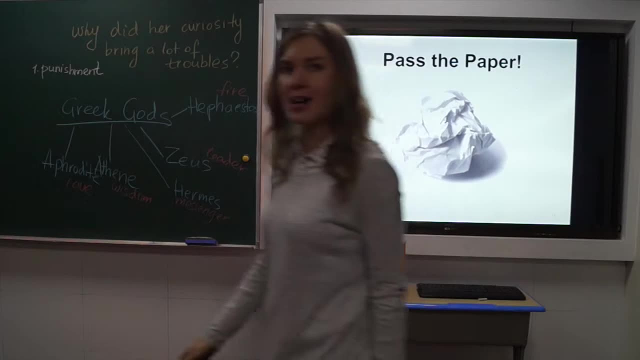 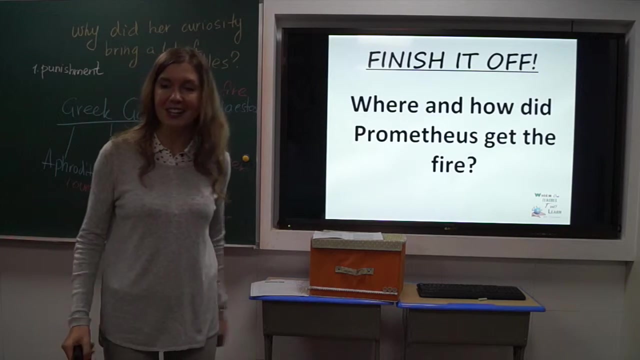 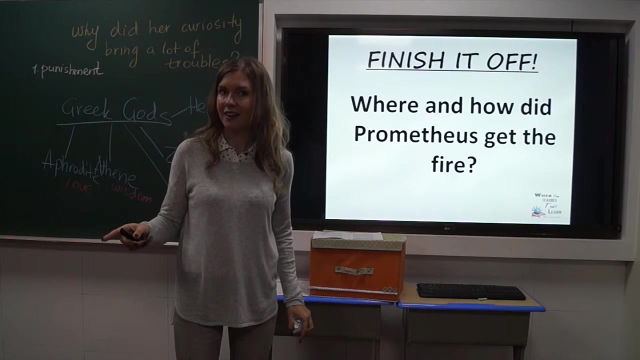 stops. please stand up and answer the question. Ready Go, Pass the paper. pass the paper. Okay, read the question please. Alright, now can you answer this question? You can read your answer from the paper. Excellent, very good. Do you agree with this answer As a homework, please? I want you to copy the Pandora.